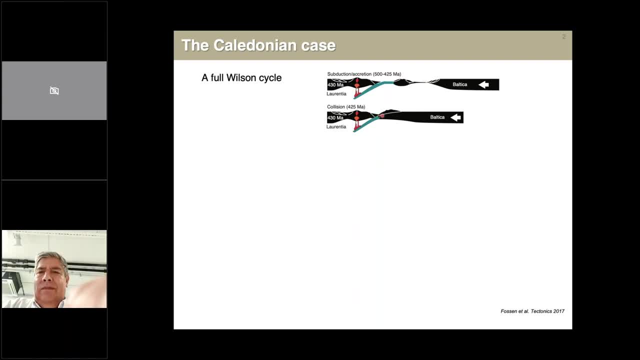 the two margins And then the ocean got in contact. the ocean was subducted and that's when the collision starts. That's the point of continent-continent collision. In the Caledonian case, that was about 430 million years ago, or 25 or 30.. 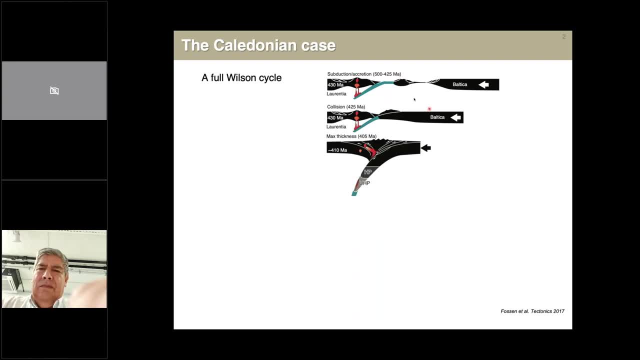 And then starts the subduction of the continent, one continental margin under the other, and the formation of the real origin, which is the ocean, and with the high mountains and all that exciting stuff. and then we get into extension, post collisional extension, maximation, and if we want we can go on in time until we form the new ocean. 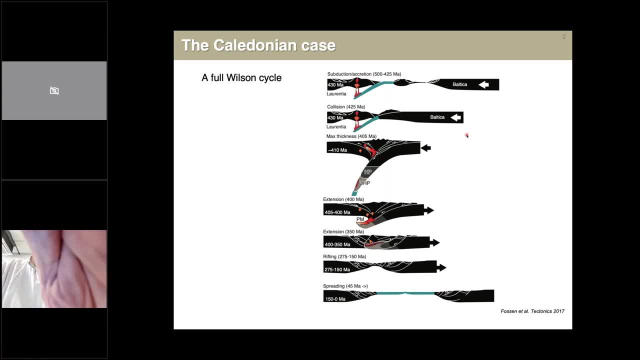 which is the atlantic ocean. so this is a whole cycle very pretty well defined, and what we are going to look at is this central part here: the time from the collision until you get so not quite back to normal crustal thickness, but sort of almost at least. 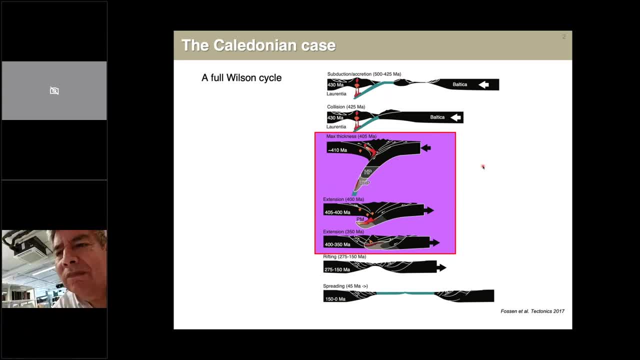 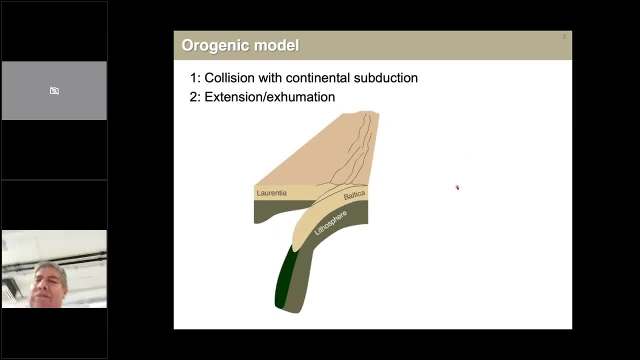 and i. there's this animation that i made at some point. we have the two continents right, baltica, laurentia. they collide, trust maps developed and then the whole thing normalizes in terms of crustal and lithospheric thickness. so this iabitus. 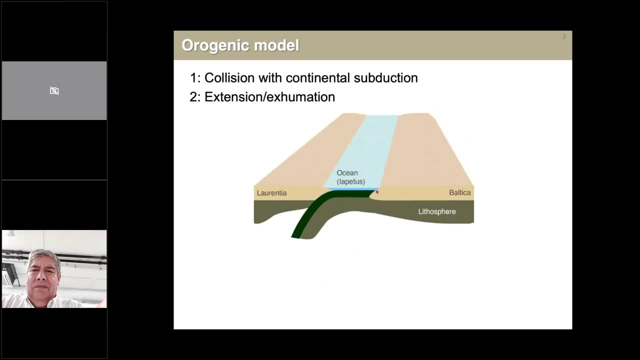 ocean that was there is going to close. the two continents collide and one margin goes down, deep down under the other, and that's a baltic and margin that goes down and then it comes back up again because today we can see these high pressure rocks at the surface. 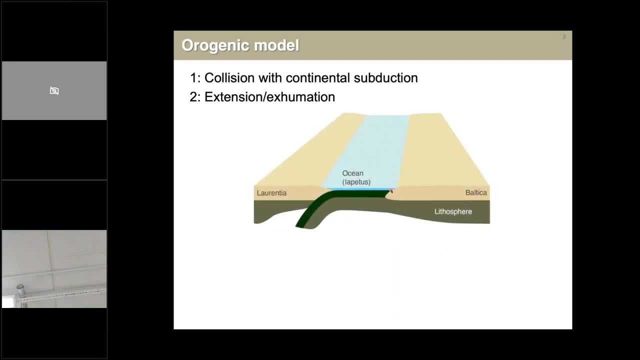 so there are these two things that i want to focus on. one is the collision and the other one is the following: extensional deformation and exhumation, which is very profound in the caledonian origin, especially where we're going to focus, which is kind of this, this area here. 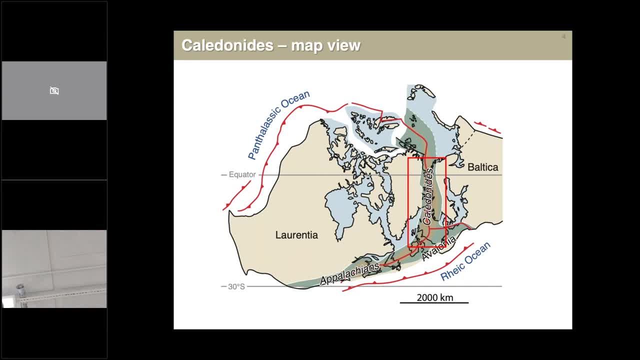 this is sort of the map view setting. we have laurentium and caledonia on the left again with greenland in particular, and baltica here with western scandinavia, norway. here these are. this is the part of the system that we're going to focus on. 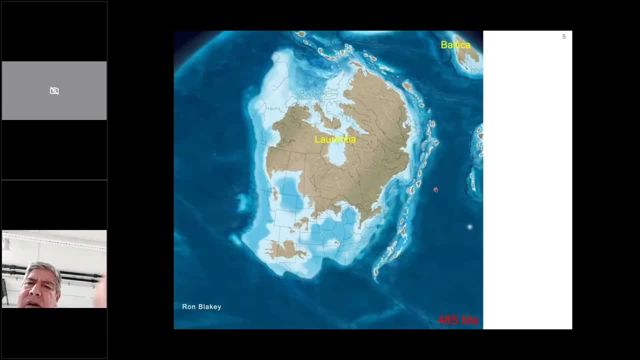 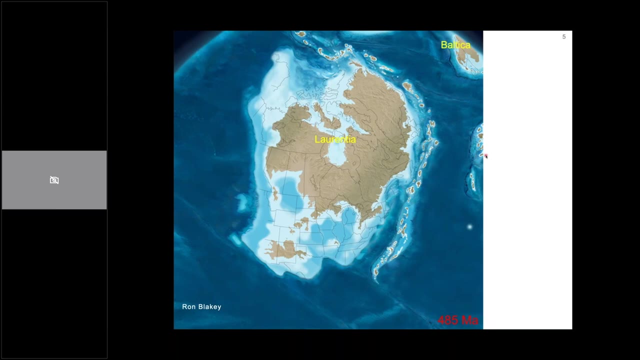 so in ron blakey's world it looked like something like this: laurentia was the bigger continent, and then baltica is over here, and in between was this ocean diapetus. so this is back in the old, 485 million years earlier division, i guess, and then this ocean closes for 50 million years. 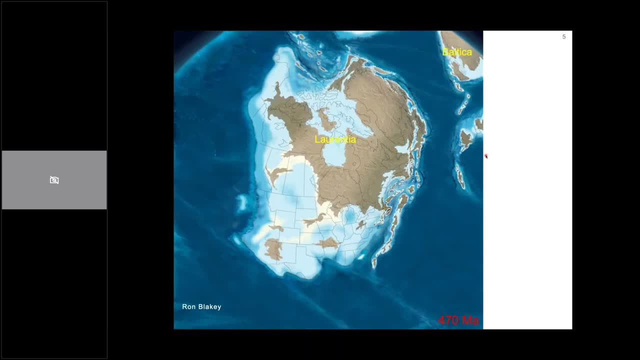 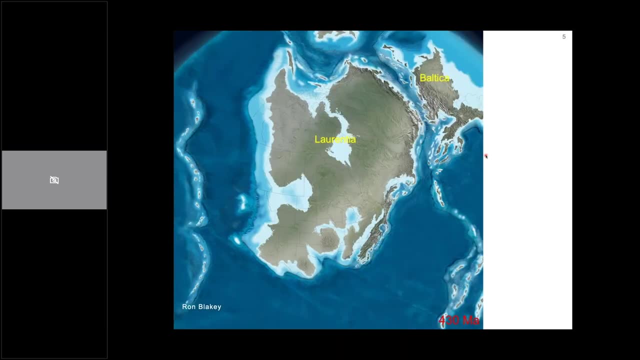 and various interesting things happen, but we're not going to focus on that. and then just to show the origin: continent, continent collision, just a little bit before 420, and you form this origin which then collapses and at that time so this is a caledonian origin. at that time, the appellation and 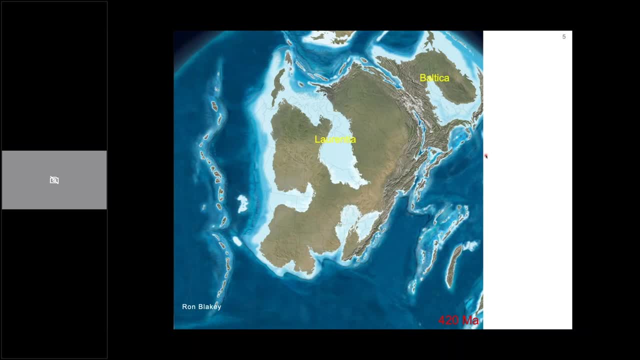 at that time. so this is a caledonian origin at that time. the appellation and the Челныthis is the caledonian origin at that time. the appellation in origins is down here and you didn't actually reach a continent-continent collision. 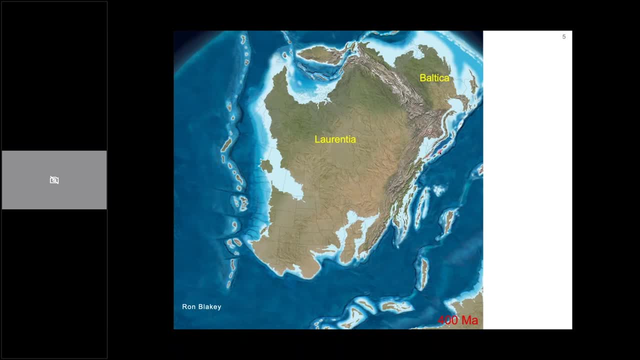 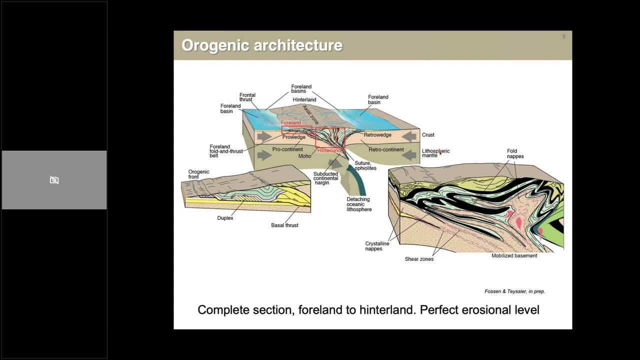 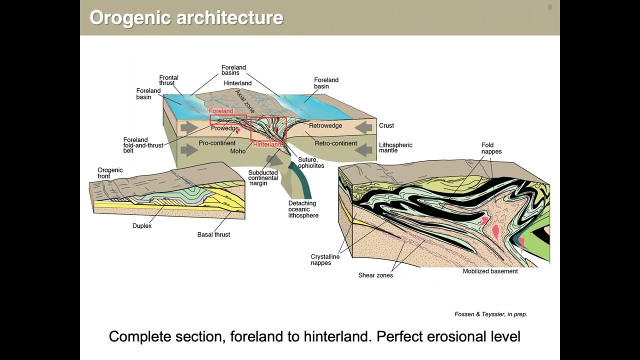 in the abolition at this stage. Okay, so it was a big origin, very high mountains and deep woods, and just since this is sort of a student setting, just to look at origins in general and look at this very generalized sketch. So we have the two continents, one on each side, and the two main components of an origin. 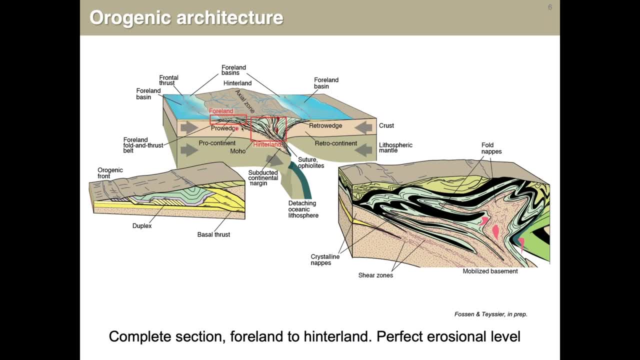 is, we could say, foreland. There are two forelands, of course, one on each side, and then there's the hinterland in the middle. there's only one of that And the foreland, you know it's low temperature, low metamorphic, even non-metamorphic duplexes and related thrust. 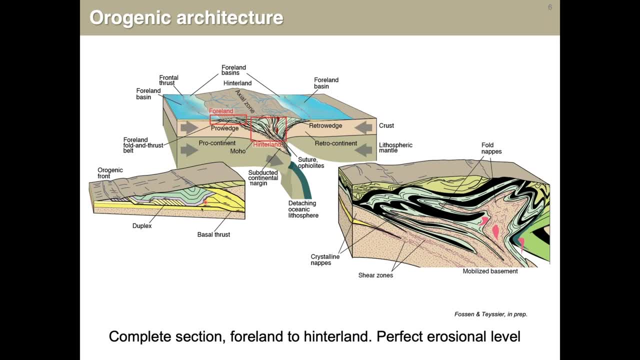 strokes. So we have the two continents, one on each side, and the two main components of an origin is: we have the two continents, one on each side, and the two main components of an origin. structures, thin-skinned tectonics, basement- not involved, at least not much, which is very 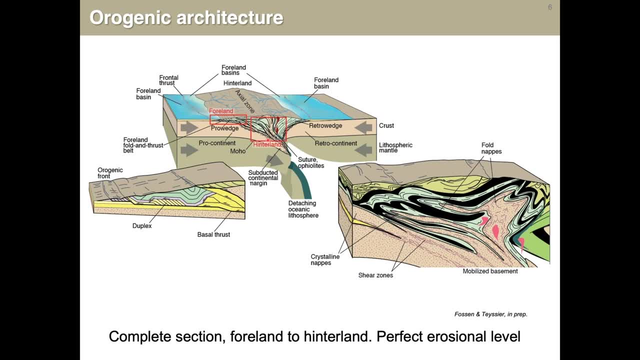 different from what you see when you get into the hinterland, where there's much more. there's higher temperature, local, higher pressures, more ductile deformation, intricate deformation and more interesting, more interesting, more complicated deformation- history at least. 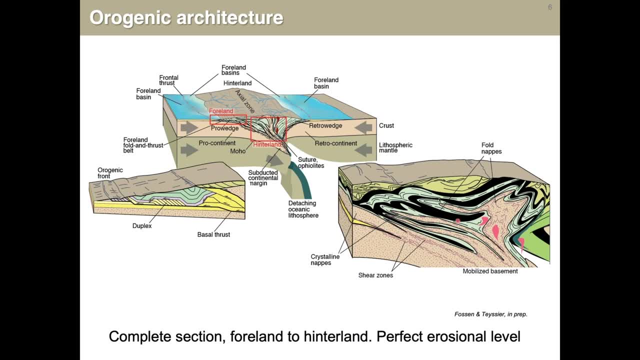 So that's the case in the caledonites too. We see these- the foreland and the hinterland- very well exposed. The caledonites is, of course, an eroded origin, so you see a various part of. 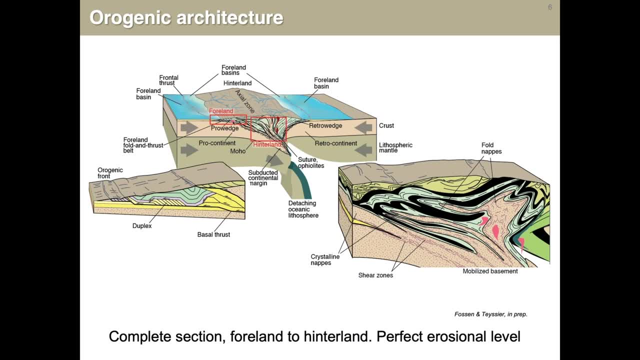 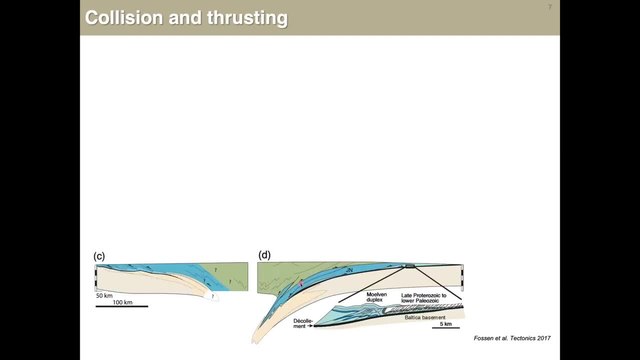 what's buried in depth in this principal sketch. So this would be sort of a reconstructed, very sort of reconstructed section, I guess, from Laurentia on the left and the Baltica on the right and, as we see, Baltica has gone down here In the right, which is the eastern. 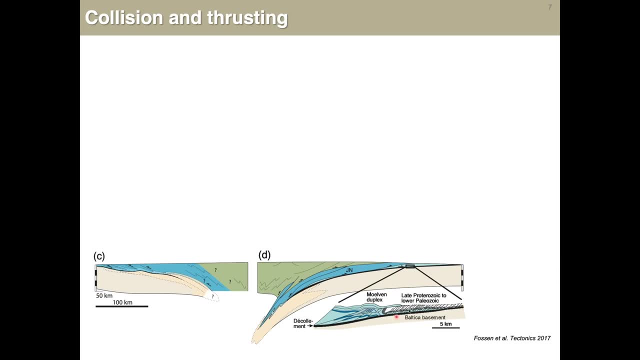 part we have these nice foreland structures, implications and thrust structures, low temperature all the way to Oslo, and this would be the hinterland in the middle right. So that's those. these are two sections, one from each side, actually from Greenland. 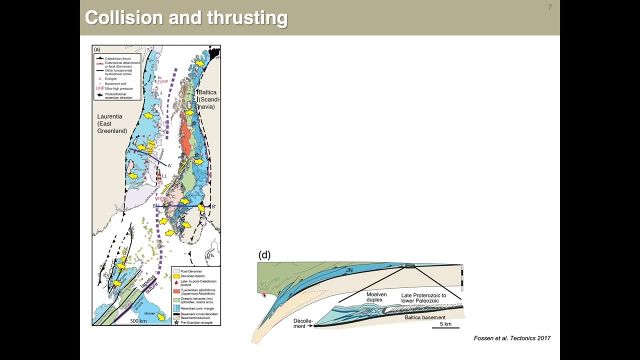 and southern Norway like this, and so this, this section that is shown now, is B- B- here in this Norwegian transect, and the yellow arrows here are sort of kinematic movement indicators or indicating the movement pattern during that collision, based on on field work. 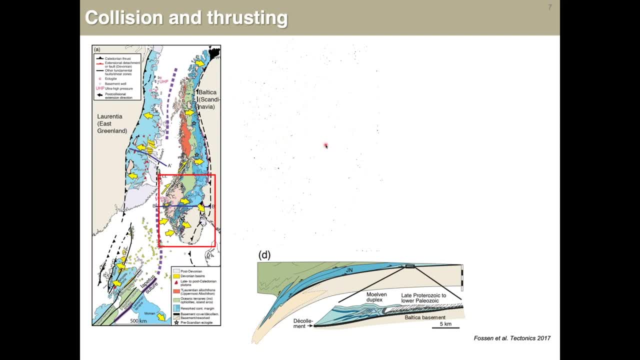 A little bit more and we see it. you see these. this is then southern Norway, and Sweden is just to the right here. So one of the things I want to show now is how pressure changes. in this section. we're focusing, then, on the eastern part, the Baltic part, So Oslo is down here. 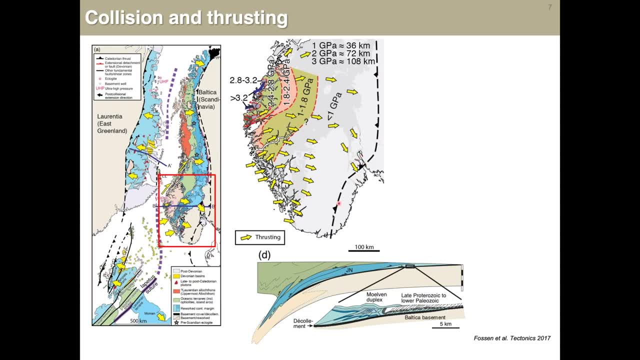 and that's sort of the frontal, the thrust front that we have indicated here. so this is a little bit away. And well, there is one one thing: there is a little bit of a change in the thrusting direction. that's interesting, but what I want to focus on is the change in pressure. 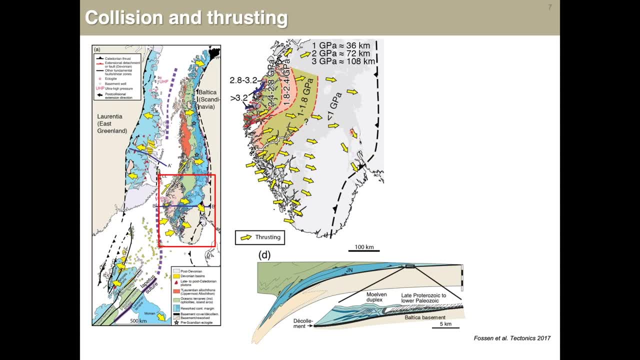 So we have, of course, a low pressure close to the thrust front. we don't have very good numbers here, but as we get closer to the hinterland, which would be here, the pressure increases. this line would be able to 1 gigapascal pressure, which is already pretty. 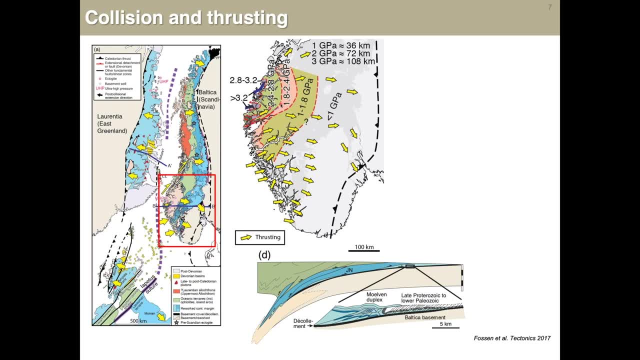 decent, and then you get up to two and three and even more than three gigapascals here along the coast. so that's a very nice gradient in pressure and these are maximum pressures recorded in the rocks. so it will be sort of the time of the deepest uh subduction, the climax, if you like, of the collision. 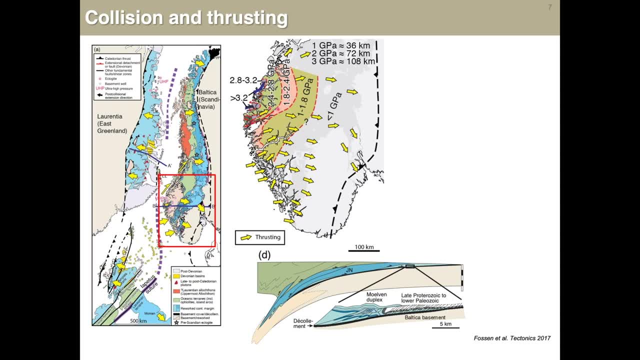 and you can reconstruct, just based on this pressure data. right, you can reconstruct what happened to the, the baltic crust, the margin, because these numbers are from, not from the thrust maps, but they are from the continental margin, the continent that was there, that was subducted. 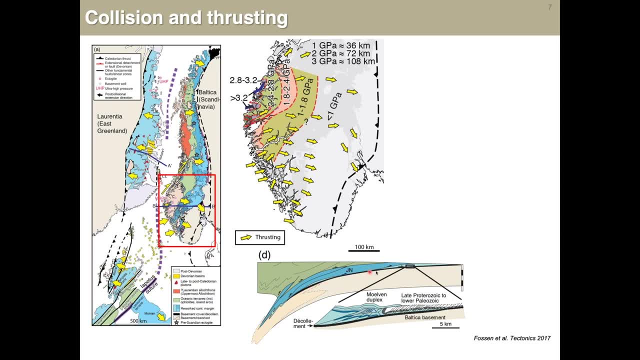 during the collision, or from the sediments that are sitting right on top of the continent. okay, and the same thing. we can do the same thing for temperatures. so as we go from move from austin, from the east, to the west, northwest, the temperatures increase gradually. so we can sort of reconstruct this sort of geometry again now. i should say that 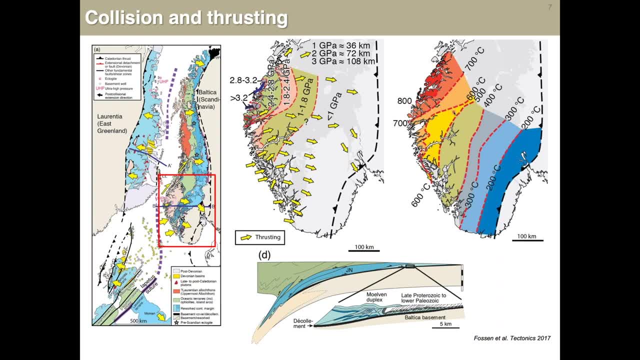 pressures and temperatures here are not necessarily completely coeval. in fact temperatures are probably a little bit younger than the maximum pressures. we get back to that. but but you get the point. we are looking at a collision zone where this part of that collision zone was um continental subduction zone basically. at least it started to subduct, of course. 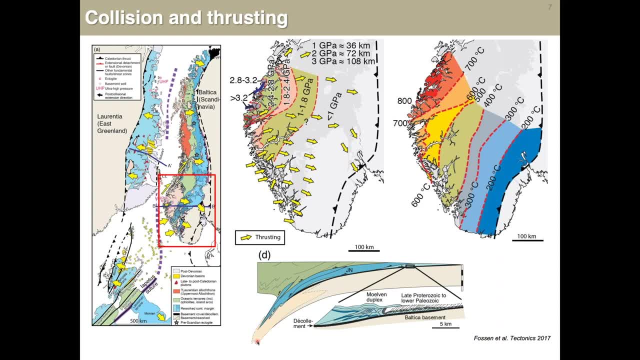 you can't subduct the continental margin. uh, very deep. we can subduct it fairly deep, as we will see from, as we see from these numbers. so out here we're talking about more than 100 kilometers of subduction depth of the continental margin. we can't subduct the continental margin at all and we can't subduct the continental margin. 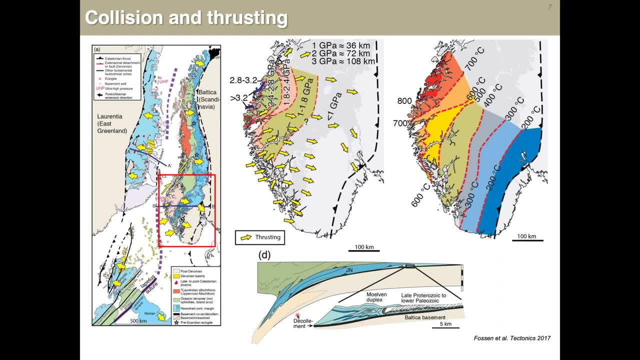 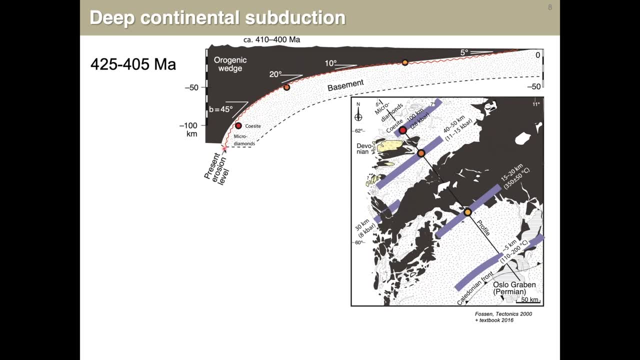 and we can't subduct the continental margin at all. so that's another sort of construction- is from, especially from from a couple of different places, how you can sort of reconstruct the base ment at the time of collision time, when it was recording these high pressures with. 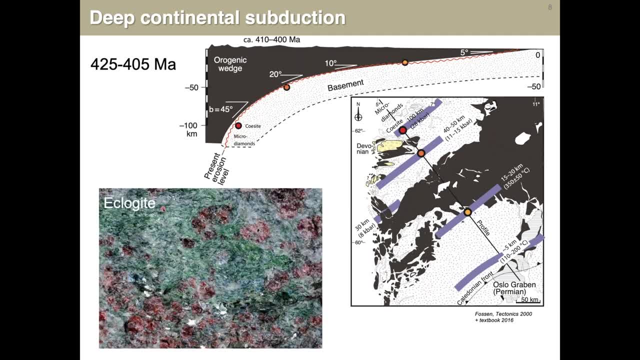 co-site micro diamonds and some really nice high pressure rocks out west here. it's a nice acroguide locality here and this, so it's important to stress that these pressures and temperatures are from the basement micro diamonds we find here. it's, you know, echo guides oftentimes are. 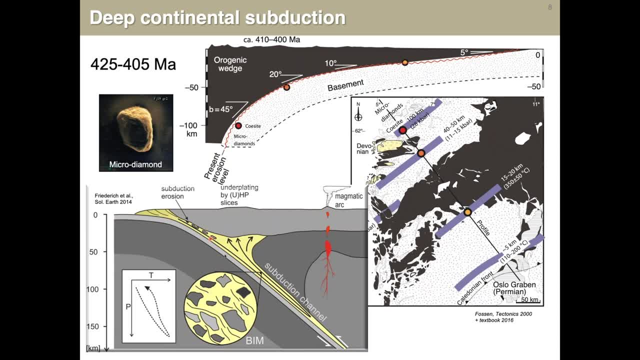 associated with subduction zones, with the oceanic subduction right and you get high pressure conditions down the subduction channel and you get that sort of return flow up and echo guides coming back up closer to the surface. this is that's something, something different. this is. 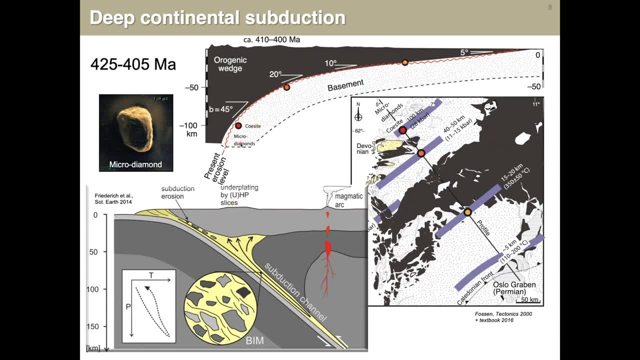 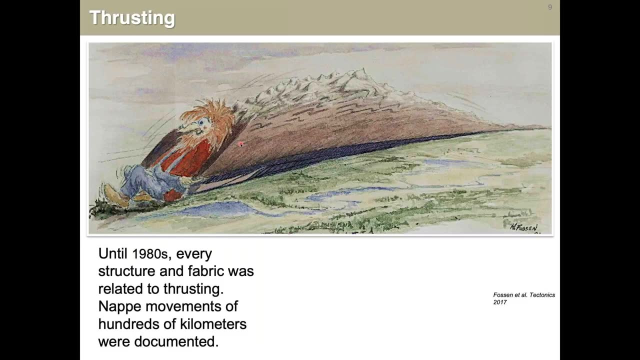 this is the basement itself during continent, continent collision. that is brought deep down and then it comes back up again. we haven't reached that yet. so we are in norway and here we. we like to think about trolls. at least we did in the old days when we was thinking, trying to. 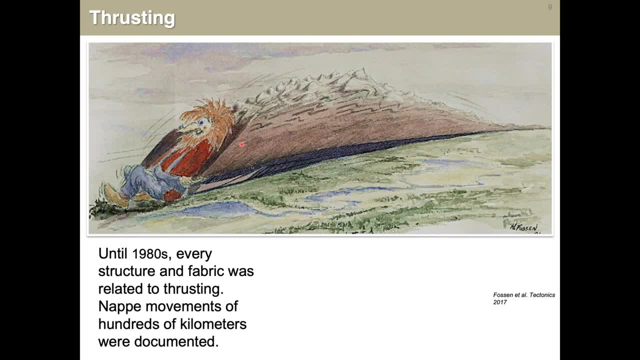 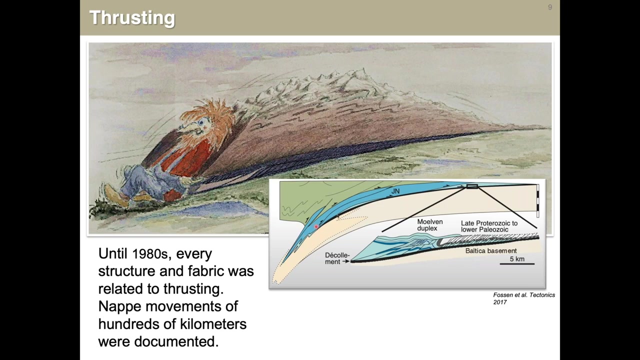 explain things in nature. it wasn't so easy to explain, so one put some trolls in here and this troll here is doing the thrusting work. right, this is what happened when the collision was going on: the pieces, fragments of of the crust and whatever was in between these two continents, these pieces were with thrust. 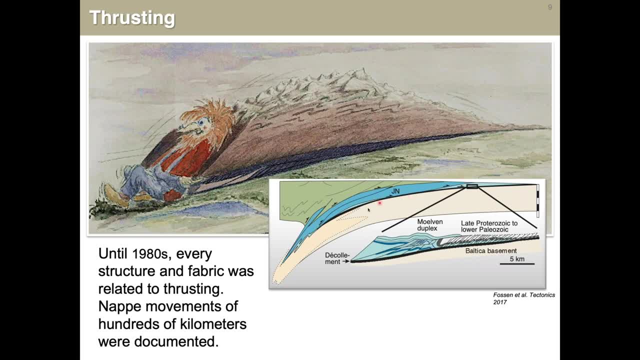 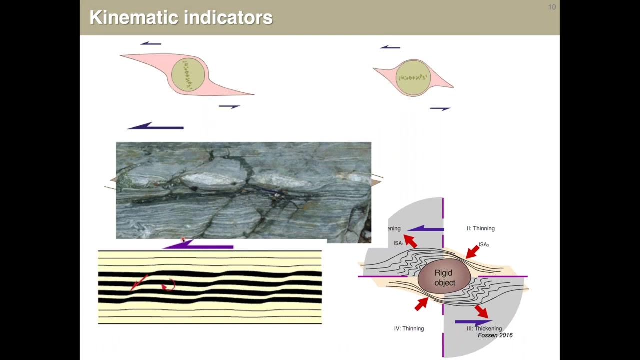 east. so these words on top of the down going continental margin of baltica. so that's nice. and when i was a student, this was all. all the structures that you could see in in the field were attributed to, to thrusting and thrust movements. then came the kinematic indicators, and this was in the 19 about 1980. 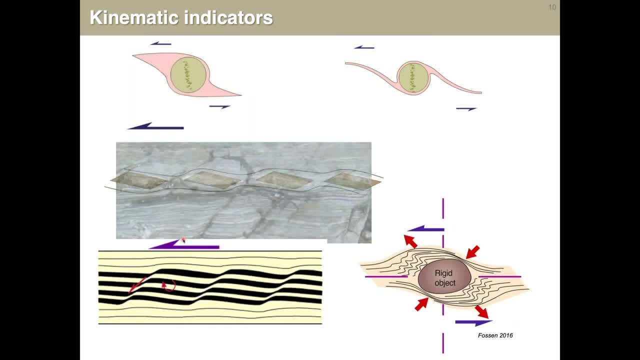 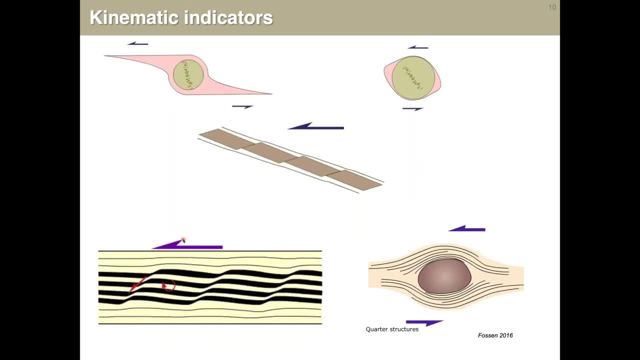 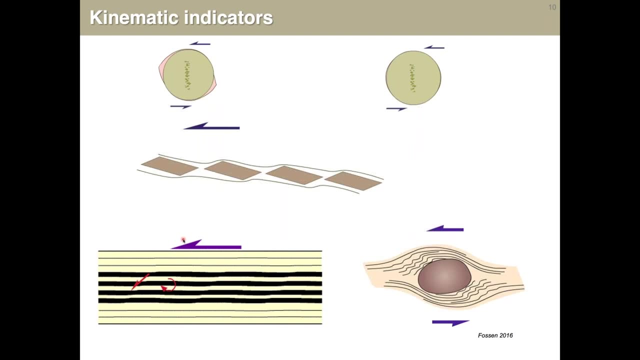 we started to understand kinematic indicators much better, with hair bands, asymmetric booleans, all kinds of asymmetric structures, and that was a major breakthrough and it changed our understanding of shear zones and thrusts and high strain zones in many parts of the world, including the calvinites and in the calvinites. 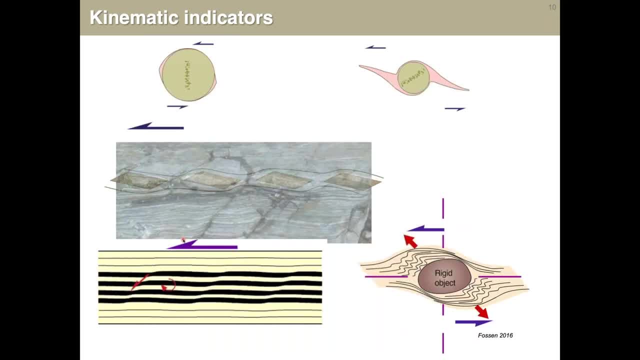 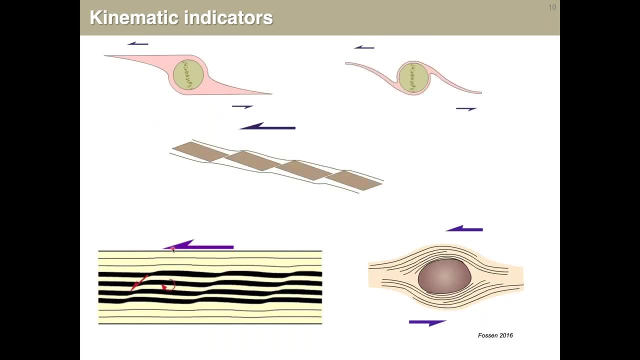 it turns out that most of the structures and all of the the obvious structures that we first would encounter if you go in the field and look at the rocks, would indicate the wrong sensors here It would indicate transport not from the hinterland to the foreland. 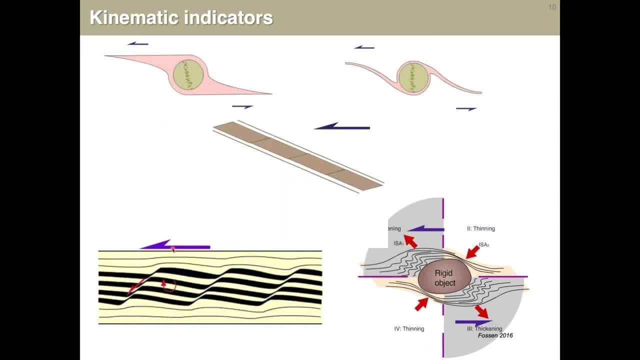 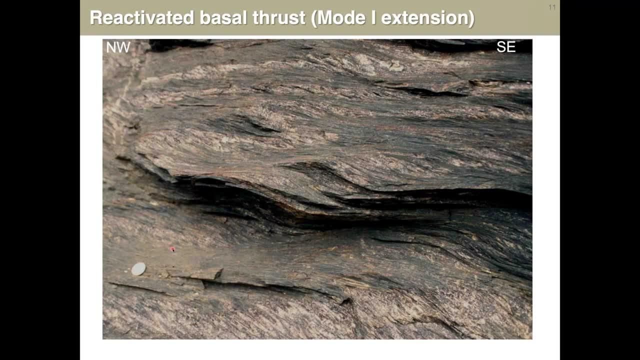 but from the foreland to the hinterland. Just a field example to show at least one couple of field photos. This is typical SC structure and you can also see asymmetric folds forming fold trains here and it's all verging to the northwest, toward the hinterland. 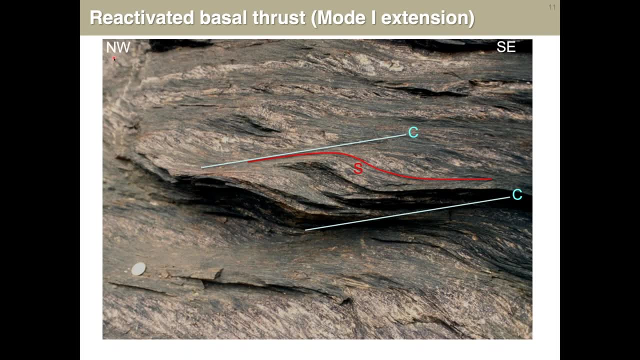 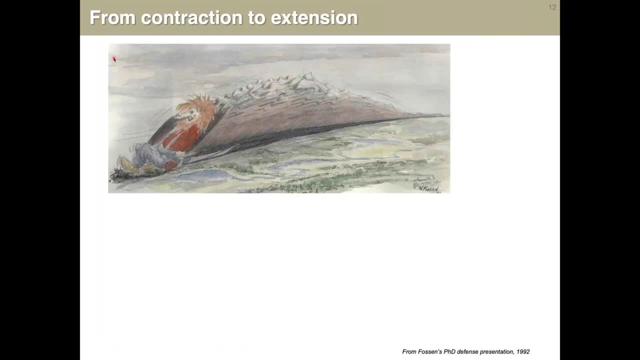 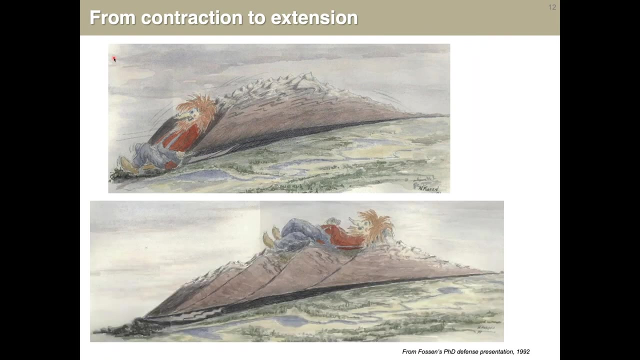 So that's changed things, changed the way we understood these things. So this trawl wouldn't then have to done more than just push these rocks to the east. It also caused some some extensional collapse, extensional structures and backwards motion of this, this thrust sheet. 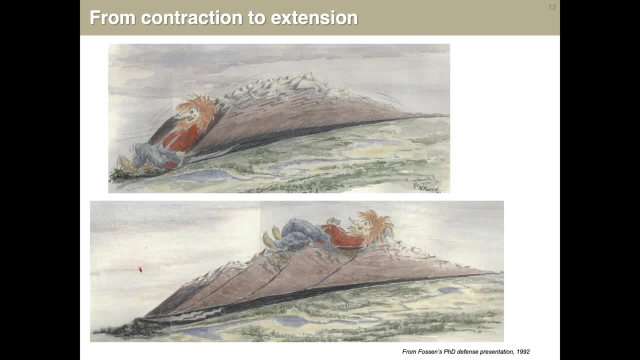 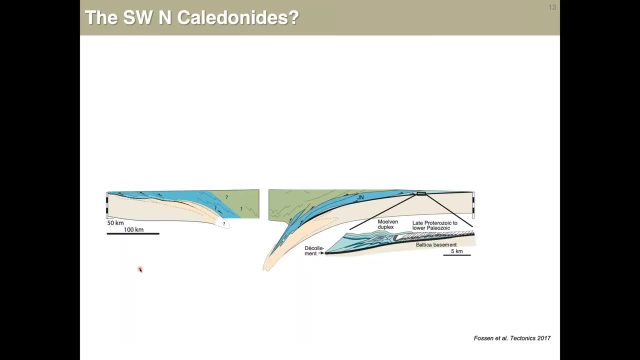 the pile of thrust sheets here to the northwest, which would be to the, to the left, And so let's see, here I showed this sort of reconstruction. If we look at the section today, it looks like this: So the difference is, of course, all these red lines and also 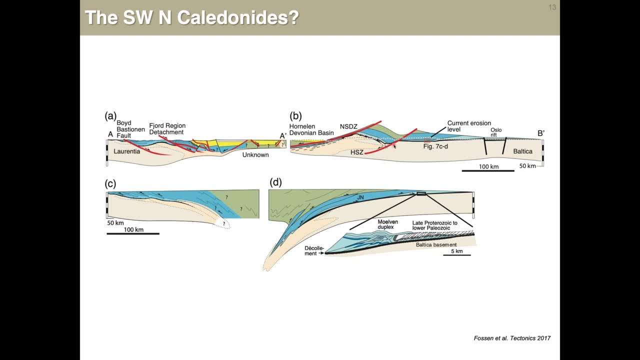 deformation along this black zone, here, these asymmetric folds, And this was sort of the figure field photo I showed from from this part here. So a lot of extensional rewinding is happening here. So if you look at the bottom of this section you can see that the 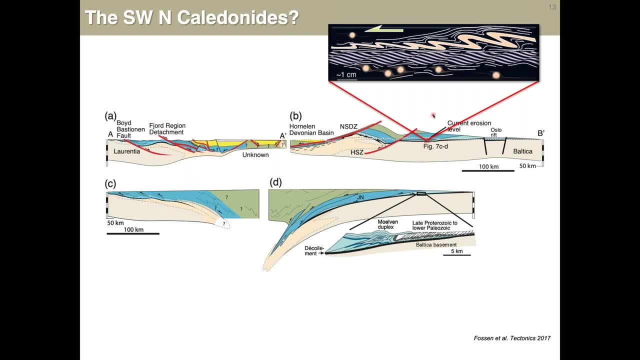 working. you go there and look at that And origin and what you- if you understand kinematic indicators and things that most people do these days- and what you, what strikes you, is extensional deformation. It's the wrong sense of cheer relative to the collision. 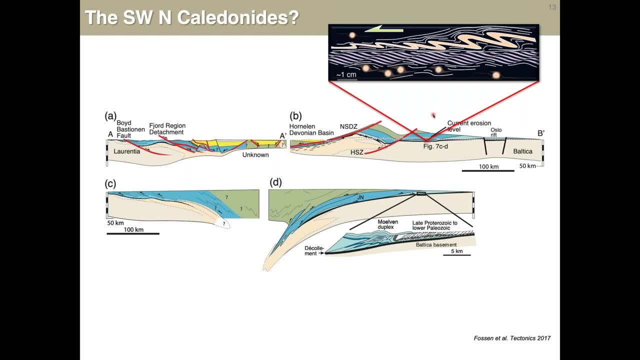 So then let's go back to this map. So this was the map showing the first thing, direction right, the transport direction, of first maps Opposite on each side of this sort of this side, this sort of deflection map. This map shows the distance line between the Yep, this is, this is, this is the, the distance line between the two sides. So the distance line between the two sides. And then when the black line and the black lines extended away like this, these were a little bit, a little bit forced into the next. 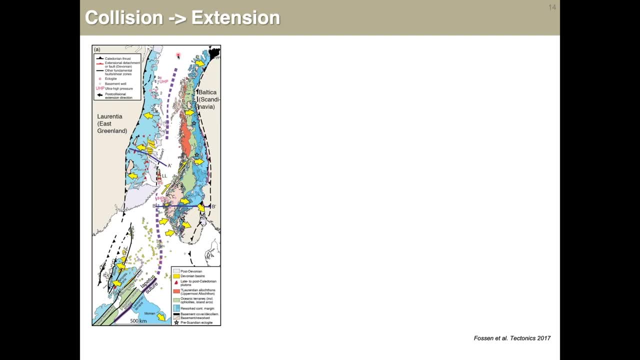 line to the left. But then you have this sort of extension left here, And then this sort of suture which we cannot really see very well today, but it's somewhere in this region, and then we can put on the extensional structures. so again, this is to give you an. 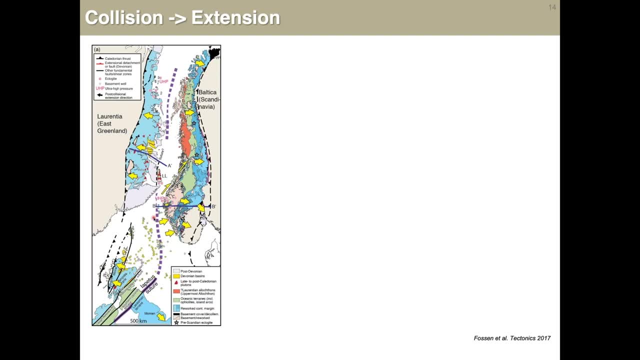 impression of the very profound extensional reworking of that orogenic structure that formed during the collision, very, very perform, and i have not seen really anything exactly like this and there are similar things, but this is very, very profound, very strong. this origin right here and especially in this region that we are focusing on here. 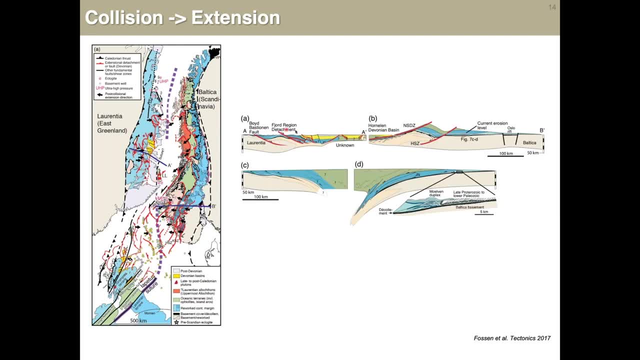 so here's that section again. that will be the same section now, from b here to b, prime. so that's a little bit this one here. this is the same section. this red line here would be that one. and then there's another one, northfield, and as the disease. 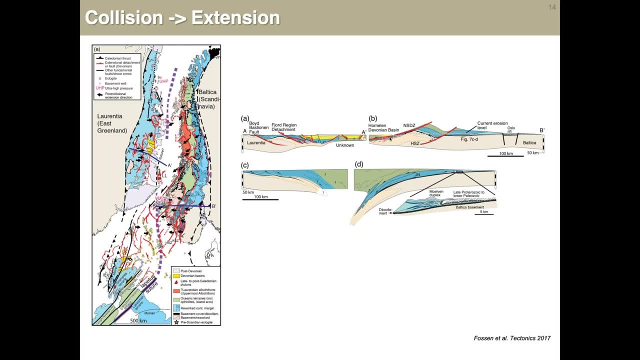 northfield song attachments on here: very this, this attention maybe 100 kilometer displacement, shear zones, the biggest ones. so we go back to this animation. now we pay a little bit more attention to not only the collision with the thrust maps but this whole history which brings that route back. 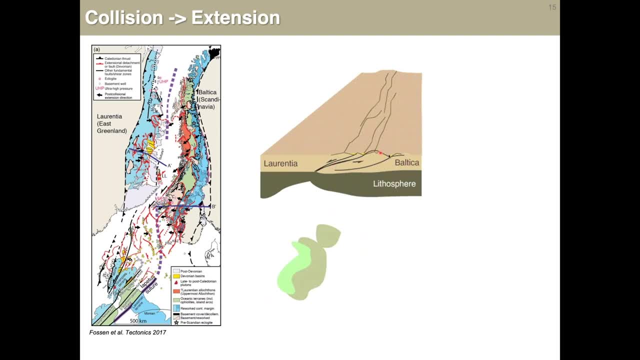 up close to the surface, uh, by extensional deformation and exclamation. so one more time: motion closing, two continents colliding and vodka going down high pressures, and then it comes back up, it heats up too and we get this extensional framework that is very profound. so so the baltic margin, the continent margin of this continent, went deep down. 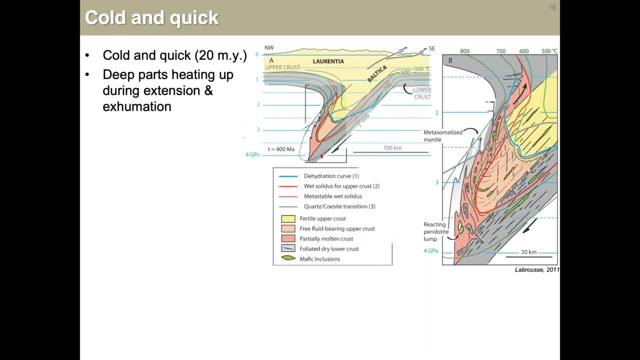 it must have been relatively cold, relatively strong, and it also was fairly quick, in the sense it didn't last that long. so it came down here as a relatively cold unit. it must have, because otherwise it wouldn't have been able to reach these depths. and then it started to heat up, and then it started to heat up, and then it 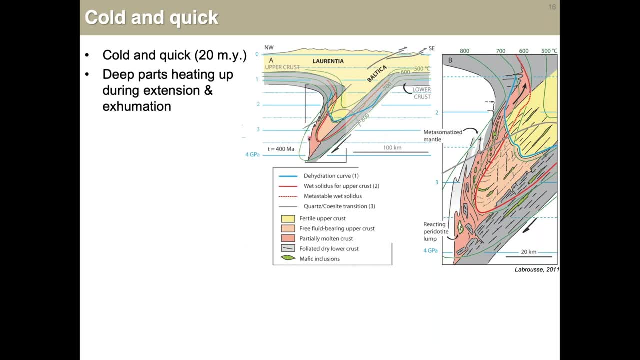 got down in the warm, deep month mantle it started heating up and that was actually actually most profound during the extensional and exhumational history. this is a figure from labros showing that we get some, some melting and things going on at the depth, but the large 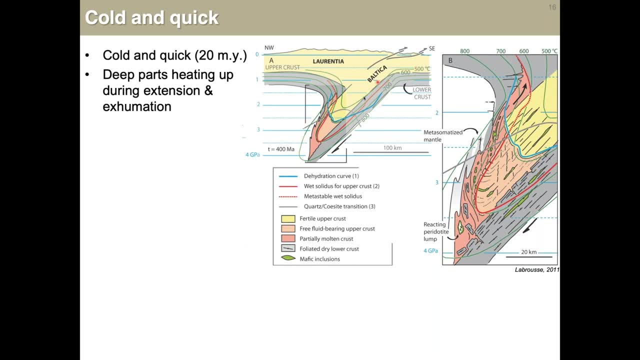 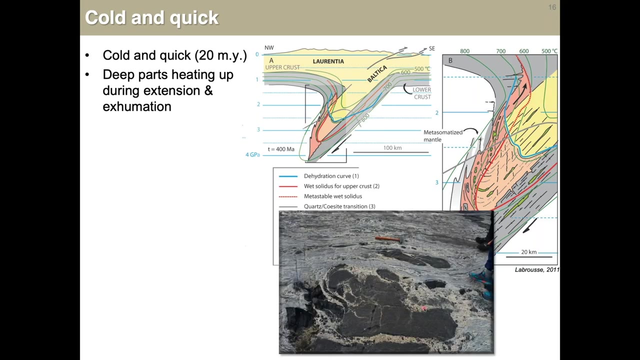 you know, enlarge this, this, uh, this margin was going down in one piece, we believe, And here is some example of melt forming in the toe. so the frontal part, the deepest part of the Baltic margin, So there is definitely excess melt there too, even though this is an interesting place. it's just in. 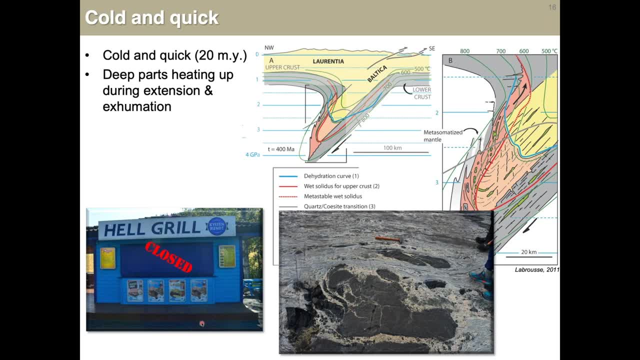 this area here. It was closed for a long time because conditions were pretty cold before it opened during the exhumation and we got some melting. So that's a place called Hell in that region, just by chance. So I wanted to show. 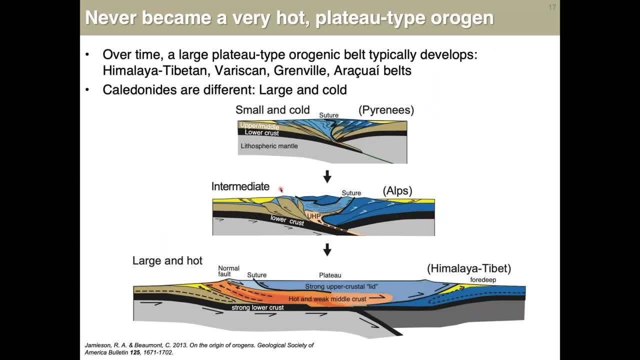 this sort of simplified but useful pattern that people, many people, think of, when, in terms of orogenic evolution, from small early orogenic until a large sort of Himalaya, Tibetan type origin. So the general way of thinking of origins is that you form a small origin and it's cold because it's not very old, basically, and then 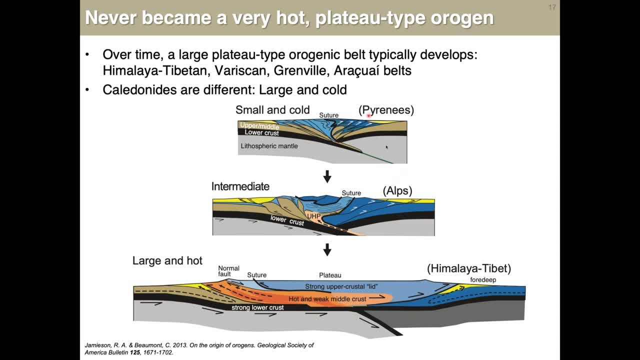 you form. the Pyrenees would be an example of that. we'll hear more about the Pyrenees tomorrow- and the Alps would be a little bit more intermediate, and then you end up in this simple scheme. you end up with sort of Himalayan Tibet, plateau-like origin, where the middle crust is now. 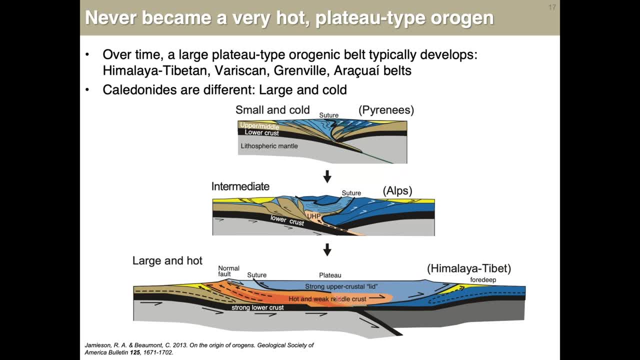 starting to melt and you have a very weak middle to lower crust, with things like channel flow occurring and plateau formation at the top, the Tibetan plateau. The point here is that the Keltonites never reached this stage. It reached the same size in terms of displacements and width, to a large extent of the origin. 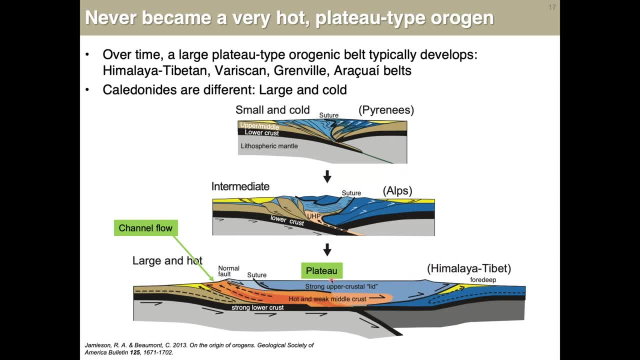 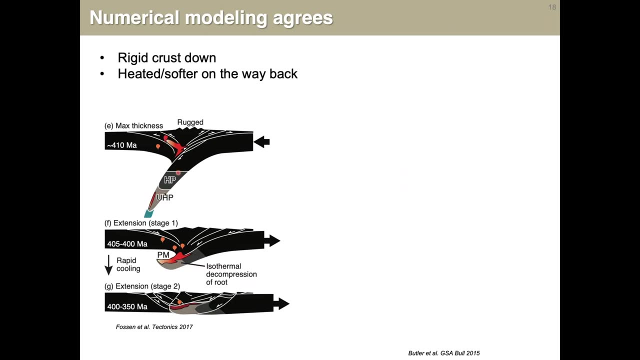 but it didn't, as the way I see it, reach that plateau stage. really, Why is that? This is basically what happened. is you put this cold slab down, the continental margin, the Baltican margin down, and then it doesn't stay there long enough before the extension kicks in, and then it moves up and 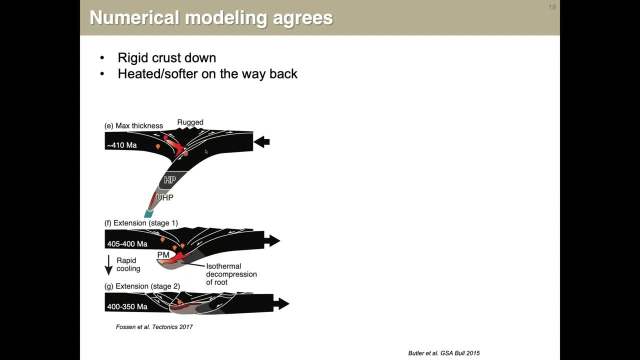 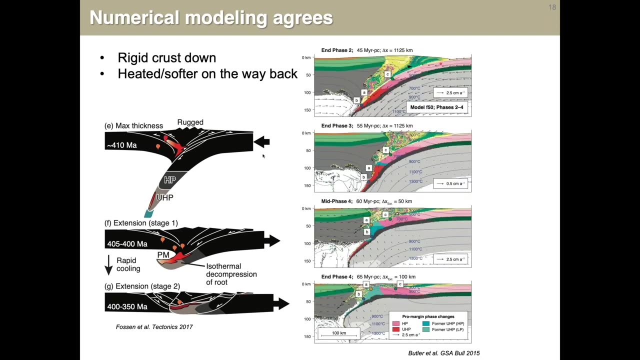 then it starts melting and then it's too late to form a sort of Himalayan type orogenic origin. This has actually been modeled by Butler and others in 2015- this model of mine here. So what they did was they put this into a numerical model. 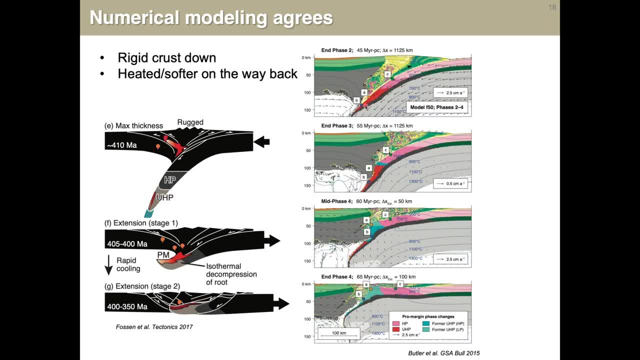 They put the continental margin down, and to do that, they also concluded from their modeling that it has to be rigid, it has to be cold, relatively cold. it goes down, and then. so these arrows indicate things are going down, right, then things change, the kinematics change and you can see this arrow here. 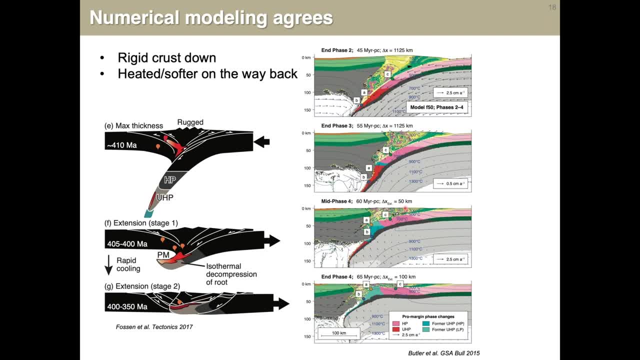 is opposite. it's the back sliding of the orogenic edifice, the orogenic wedge on top of the, the base material basement is basically pulled back, and that's called induction, the opposite of subduction. so it's first subducted, then deducted, and that's what this arrow also indicates. this thing is. 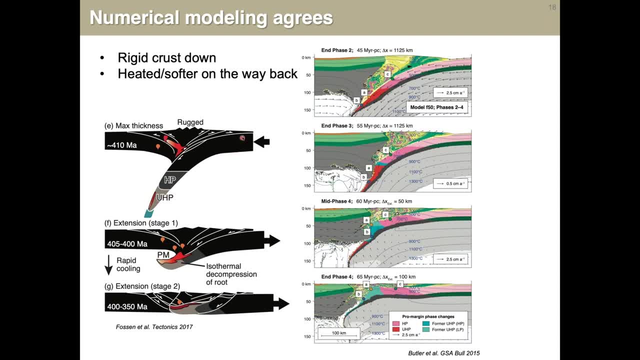 pulled back, basically, and you reverse the kinematics at the top of this continental margin and you get extensional deformation right on top of that. and then you, at the same time, you move and you assume the subducted margin. and this is interesting- you see the arrows pointing up now and you get things very close to the 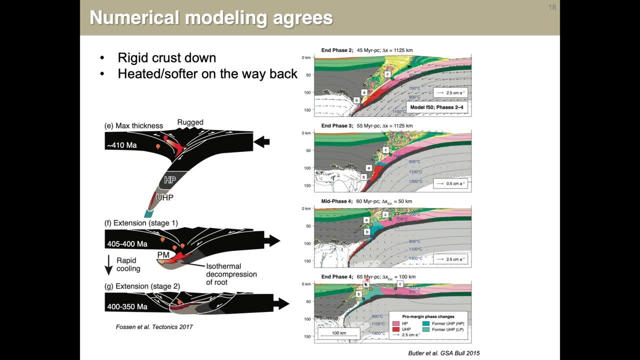 surface over a relatively short period of time- this is 20 million years between the top and the bottom. here this model, and you can in the model, you can put in these temperature, pressure or sort of model paths which show a very characteristic and clockwise right pattern, and that's what we see in the real data too. 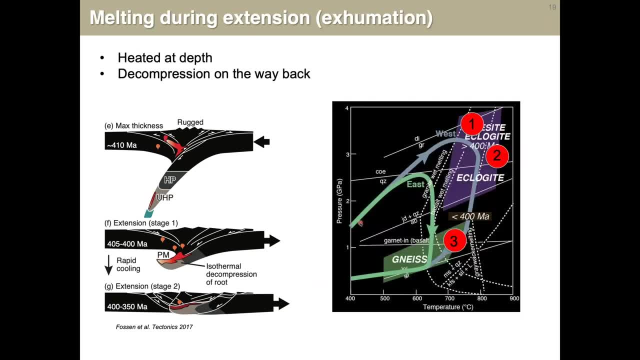 in the field data- that's where we estimate pressures and temperatures taken from many different sources- that you have this clockwise pattern. so this first path here, reaching the maximum pressure- would be the maximum pressure of the subduction right that's up here actually to be accurate. and then 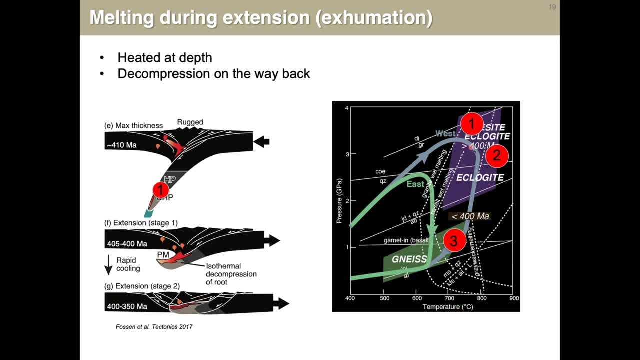 pressure goes down. the temperature still increases to the right here until about 2.2, which would be more or less here. so you get more heating and also you get the decompression. the pressure is now lowered from 0.1 to 0.2 quite significantly, which means that you more. 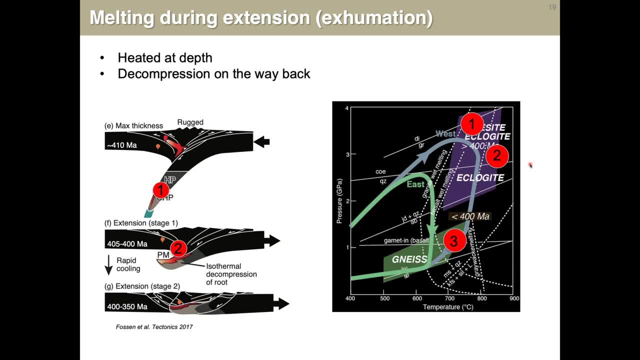 easily start to melt the rocks. and now you're starting to melting, now you're starting to soften the whole system, but it's too late to prevent this slab to go go down deep. and then three of course, in the end we get down here. so it's interesting: the melting in this origin happens on the way. 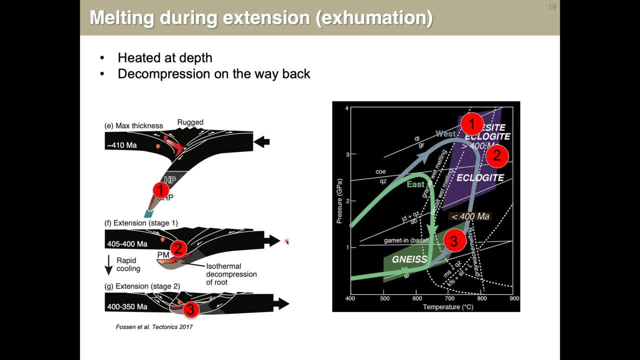 back to the surface during extensional deformation, not during collisional kinematics or convergence. so it's a little bit different. and what happens then during extension is a little bit different. it's it starts to the lower and the middle crust starts to to become soft and flexible, and we got 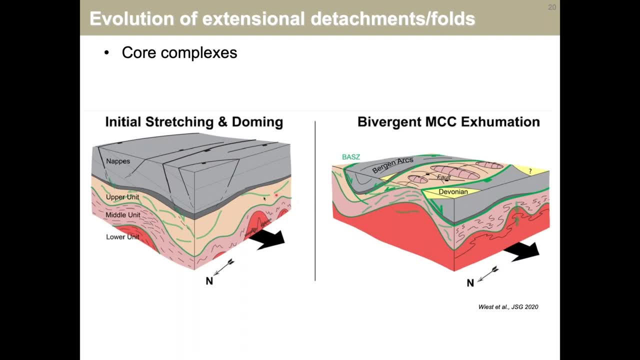 these uh sort of domes and two big folds that develop into core complexes with major shear zones on top of these core complexes and basins. this would be in the devonian, so you get devonian basins here. this is um some nice work by a recent student at the university of bergen. 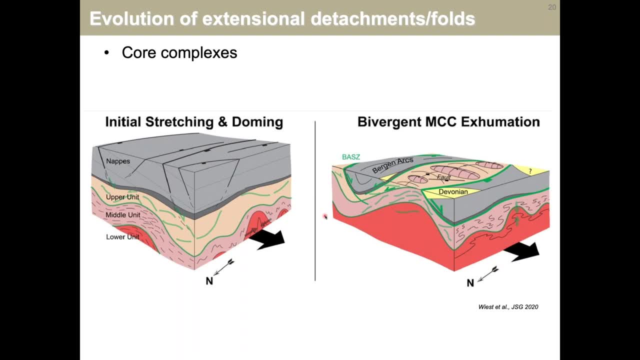 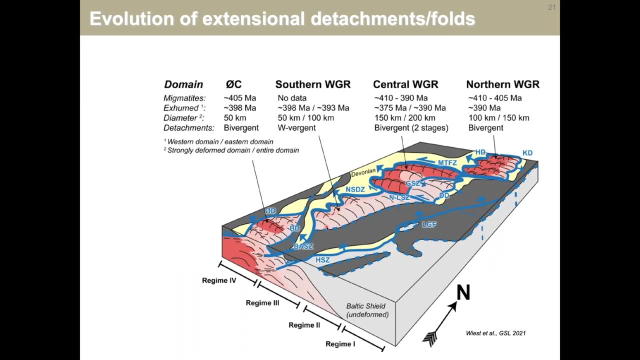 the one is west and the next figure two. we're illustrating this, so this would be the coastal area of, of, uh, south norway. so it would be this area right here, with these um things swinging in and out like that, with basins on the top and this. 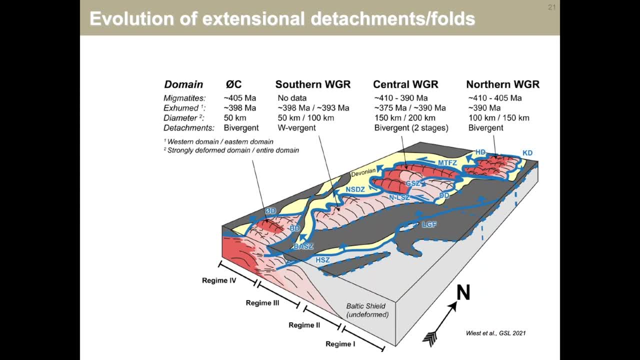 hot crust sort of you know, moving up into these core complexes that are bound by in blue hair extensional shear zones. some are very large displacements. so this melting, this is concluded from, from dating the melts, of course, in these different places and the dates are from: 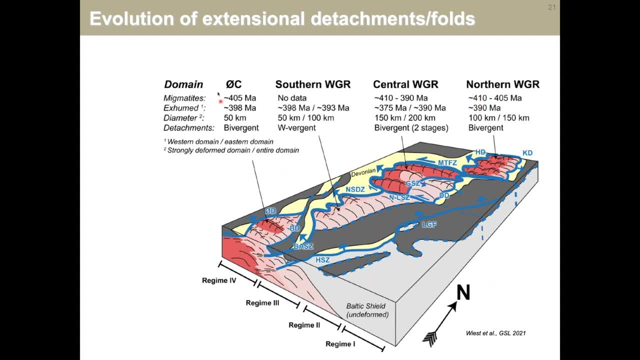 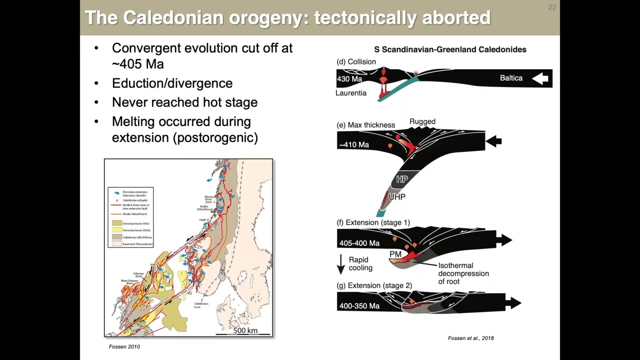 most of them, 410 to 390, 375.. so just at the end or after the convergence ceases and the divergence starts. so, um, i think a very important thing that helps explain the caledonites, in this part of the origin at least, is that the whole. 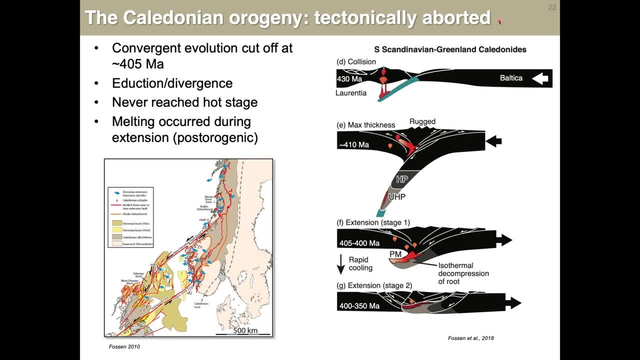 orogenic process was tectonically aborted. it was cut off at 450 million years of what we know as the caledonian had dated. that's when the whole thing was cut off and we started to have adduction divergence and we never reached the hot. 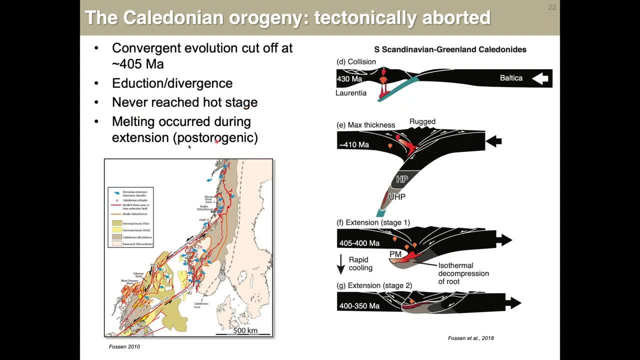 orogenic hot contractional stage, but we've got no melting occurring during extension in the post-organic stage. so not much melting here, a little bit, but then most of it during the exclamation. that's how do we explain that? well, there's one explanation that was put forward by patrice ray back in 1997. that is: 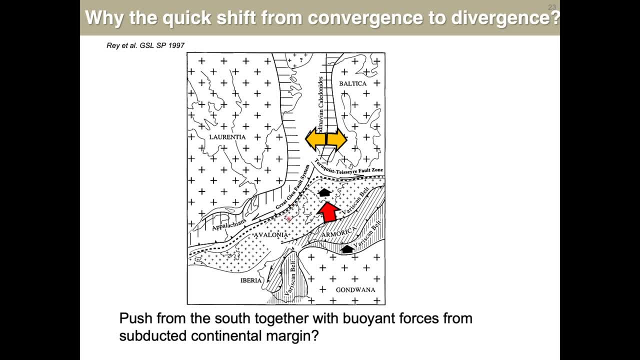 still quite interesting and that's, you know, the push from the south. there was avalonia here that seems to have been pushing northwards and with this shape here it could have started some divergent movement between um stanley navy and baltica and lower asia, so something like this right, so that.